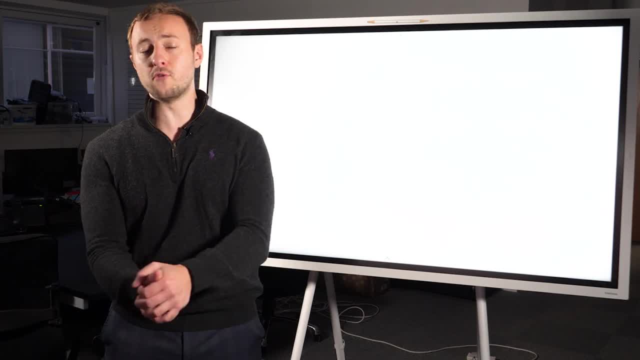 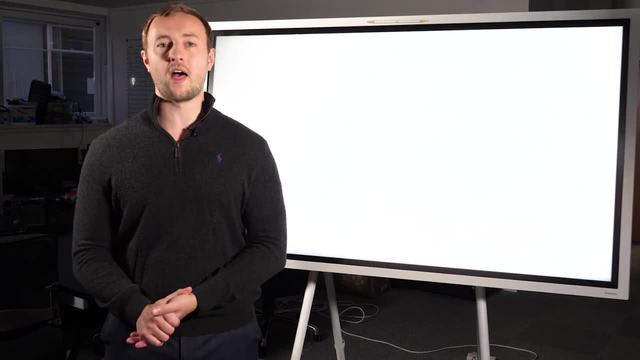 You then find a great tenant that's really grateful for you putting a roof over their head and creating a home, And then you're also going to be really grateful because they're going to pay you for the privilege of that and never hear about again. Well, it doesn't really end up like that. 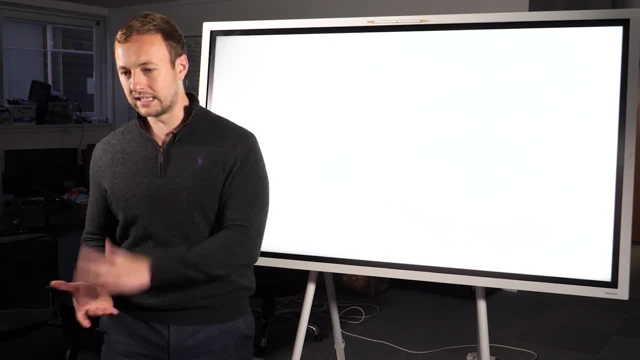 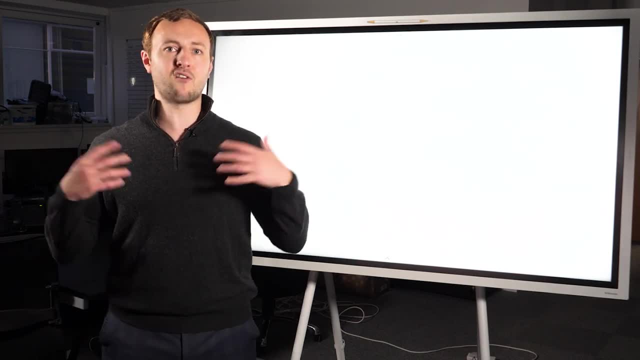 Tenants tend to break your property, complain there's leaks, there's the boiler gone, smashed windows. They're complaining about the neighbors, The neighbors are complaining about them. They have parties And, of course, the massive Doberman dog. when they asked if they 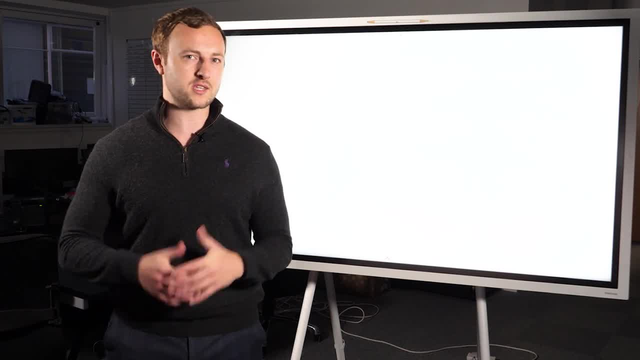 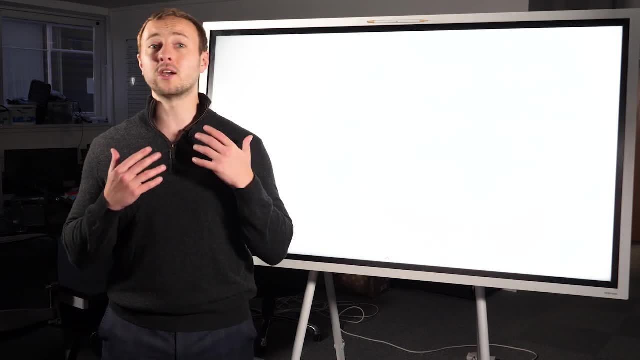 could have a goldfish in there, And that's not quite what you meant when you said pets may or may not be allowed. Well, not all tenants are like this. We actually have some really great tenants in our properties. They pay all the time. never have any issues with them. You don't hear. 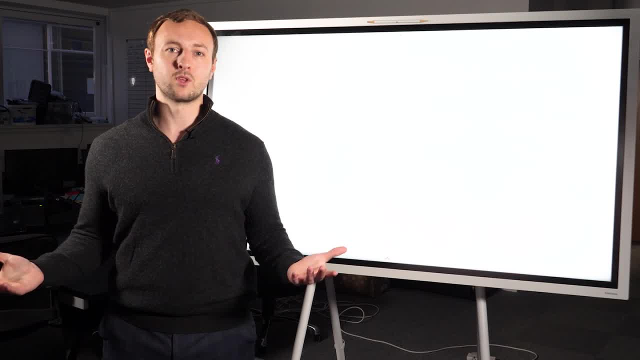 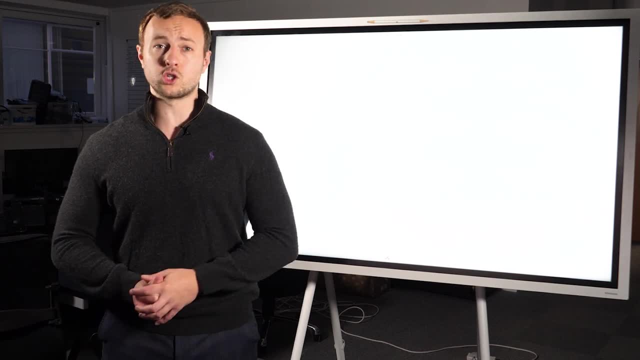 anything about it. You do your inspections and the property is well looked after. But when should you get it managed? Should you self-manage? Well, this is going to depend on a lot of situations. First of all, let's just cover the ones where you absolutely should have a manager. 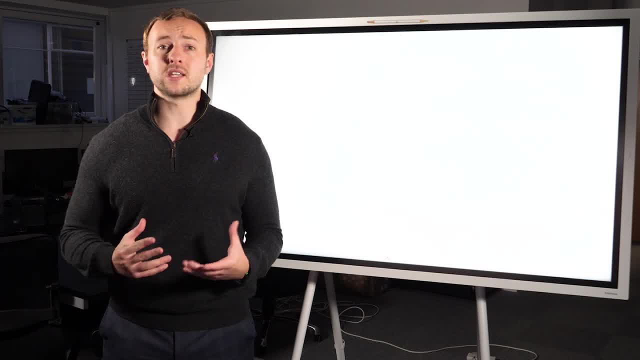 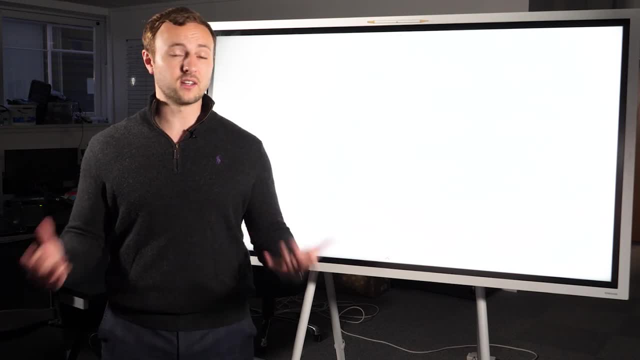 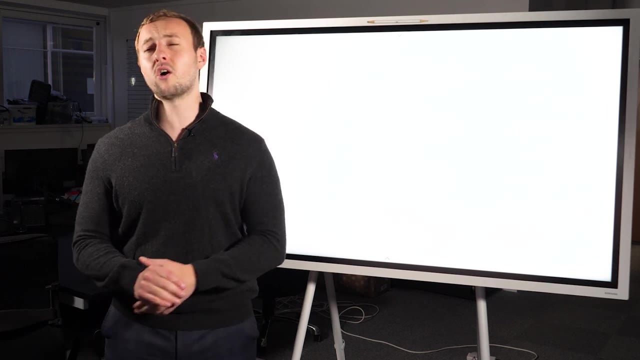 in place. If you have a property in another country- Okay, there are a lot of, a lot of our investors are overseas, from Hong Kong, South Africa, Japan, et cetera, the UAE- It makes complete sense having a property manager looking after the property, because the last thing you want 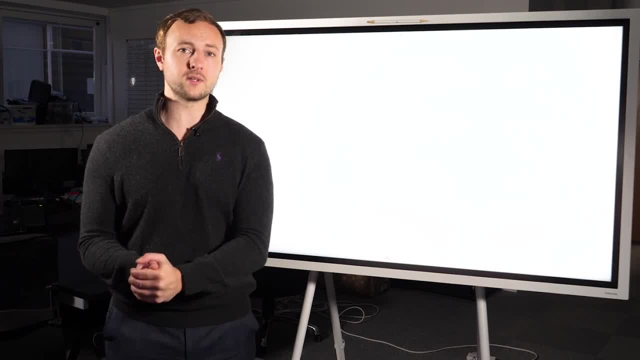 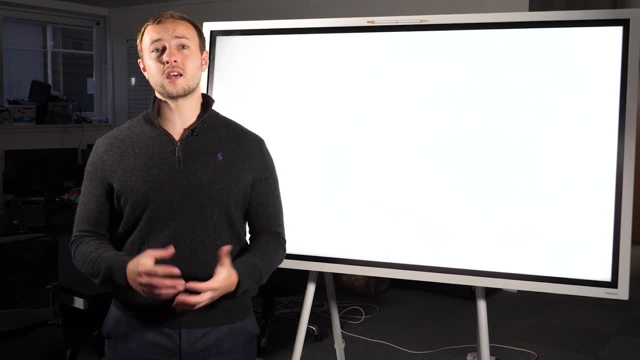 to be doing if you're in another country is getting a phone call directly from the tenant, then going: look, this has happened, You need to send someone around, and having to deal with that on an ongoing basis Goes the same, by the way, if you're out of area. 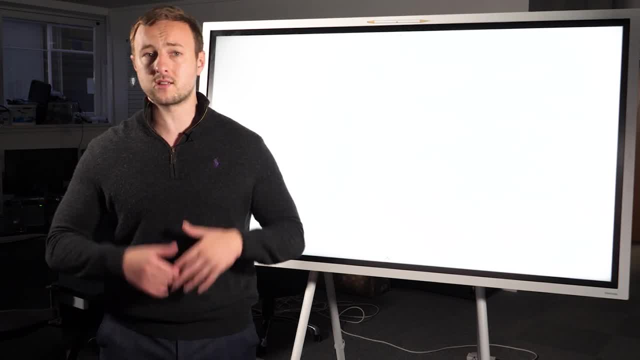 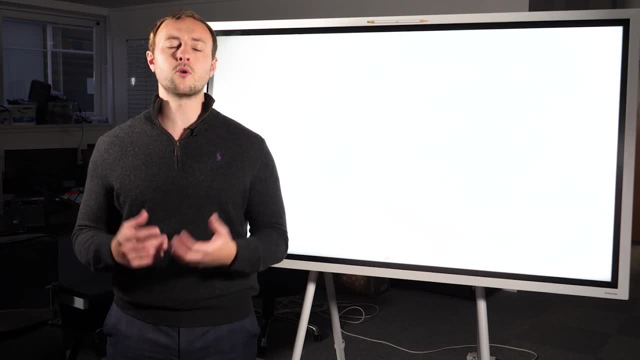 if you're in London and you're investing in Leeds- which is where I'm based- incredible place to invest, Actually, no, it's not Stay away from it- Then you're going to want a manager in place. okay, Because they're going to take care of the day-to-day needs of your tenant. And if you've 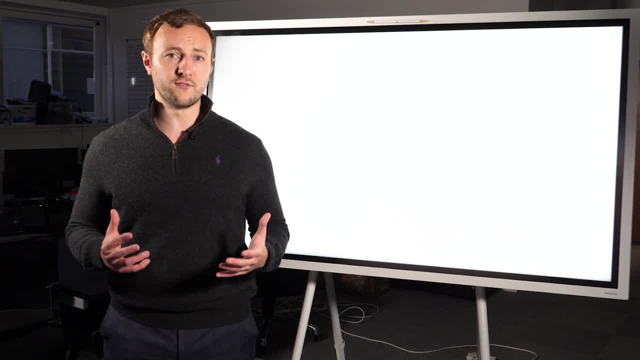 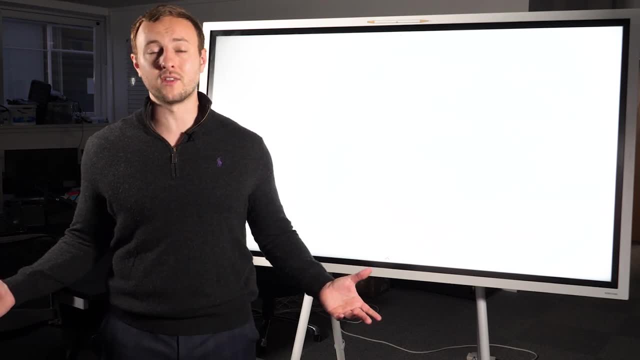 watched a lot of my video and my content. you know I talk about the value first principle a lot. I believe in adding as much value to other people And this is because, hey, it's nice to be nice now and then right. But also from a business perspective I'm a massive believer in that. if 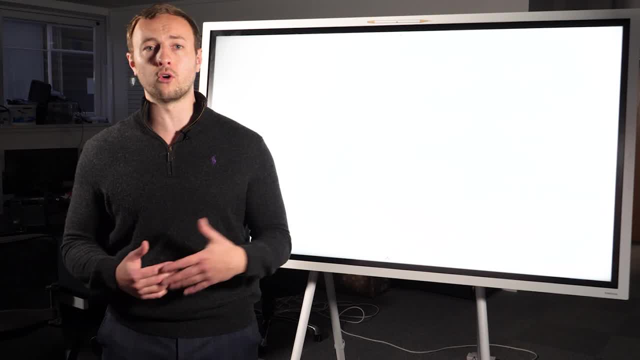 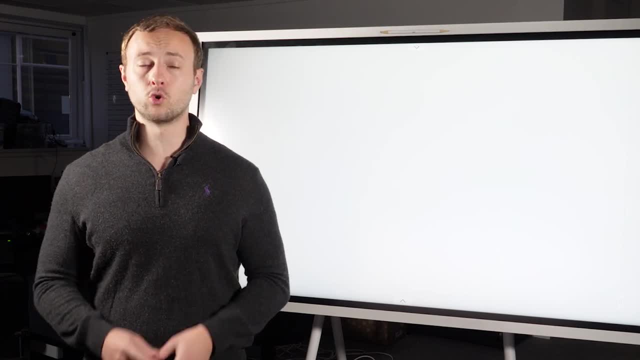 you add value to people's lives, they will tend to pay you for it on an ongoing basis. So another reason you might want to consider getting a property manager in place is if you're a portfolio landlord or you're intending to be a portfolio landlord Ultimately. 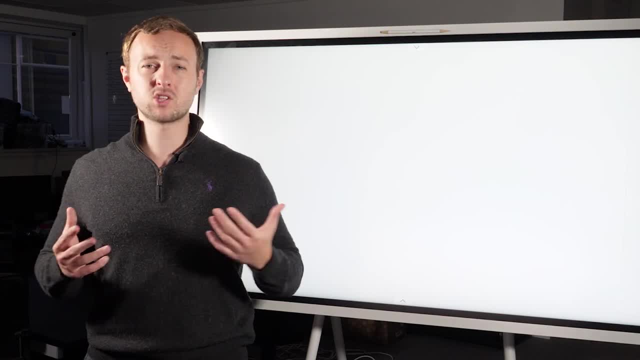 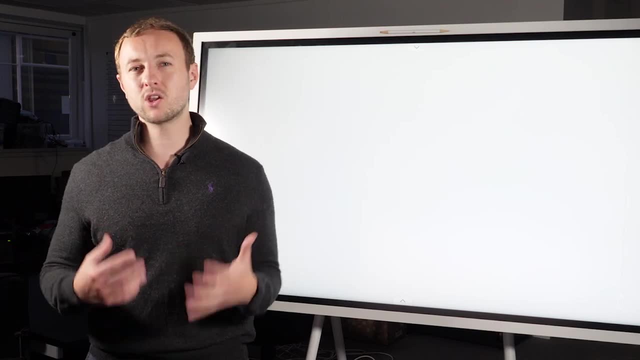 it's that time versus money principle A lot of people, when they start out investing, what you seem to value the most- and I did too, by the way- is you value the money the most. Well, as you get bigger and you start circulating, what you should realize is you can always make an. 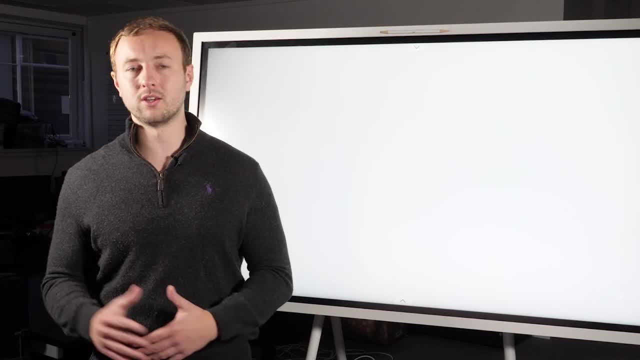 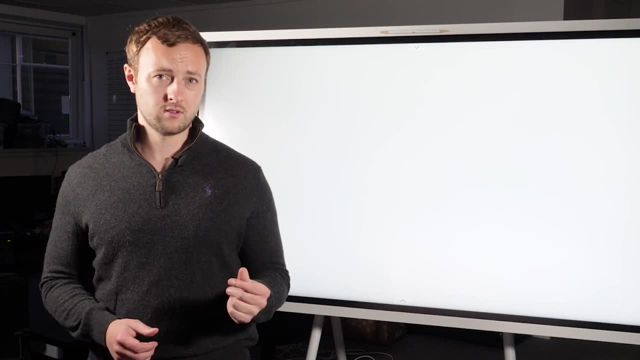 extra thousand pounds, or million or billion, maybe not a billion, but eventually right. But each pound you can earn another one. It comes and goes, But time I won't waste any more of yours is gone, okay. Once that second's gone, it's gone forever, It's. 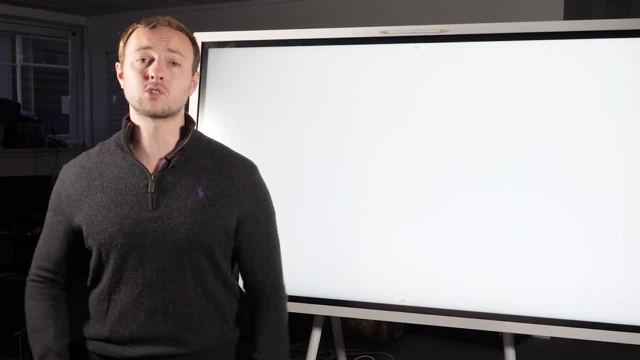 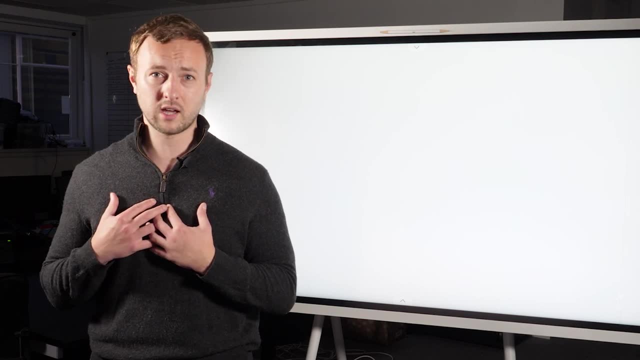 this bank that is emptying one second at a time, one day at a time, And you want to utilize that as much as possible. So for me, I'd much rather pay somebody else for their time and take away from mine, okay. Now, whilst we're talking about that- the cost of time- what does it cost for a property manager? Because there's several reasons, maybe, why you wouldn't want to get a property manager in the first place. So a typical cost that you're going to come between is 8% and 12% plus that. 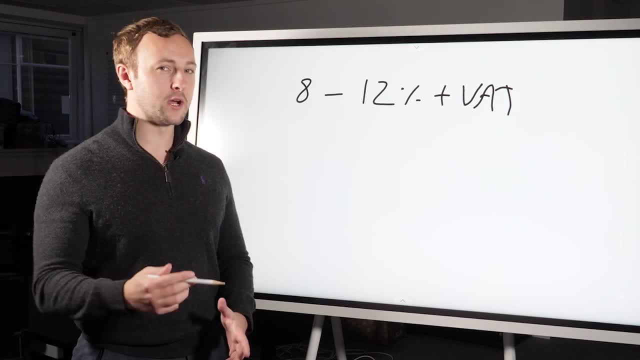 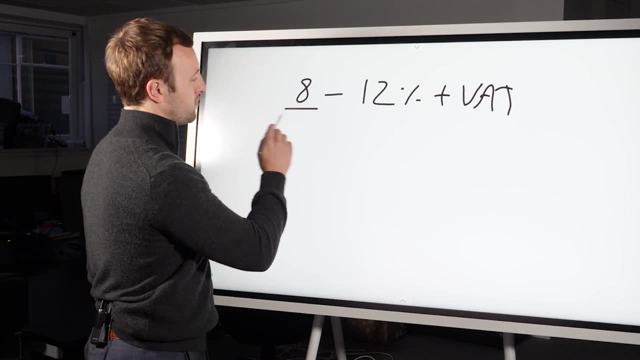 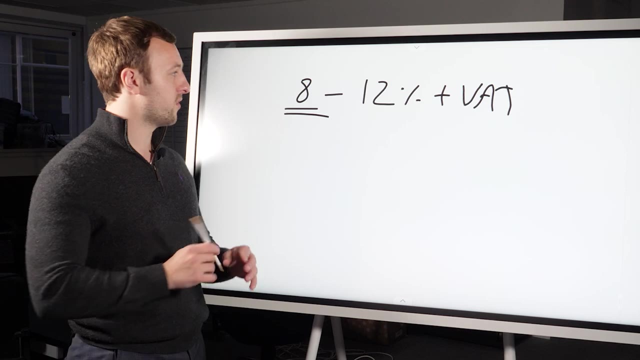 Okay, Now I'm going to break this down because I think this is really important, because people are motivated by money. okay, So 8% in my experience- I'm not saying everyone, by the way, but this is good if you're thinking about becoming a property manager, of how to price yourself. 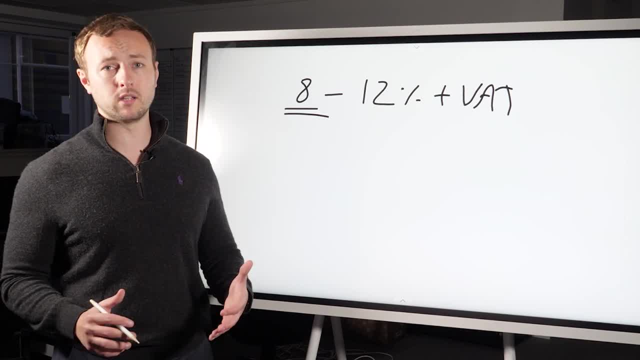 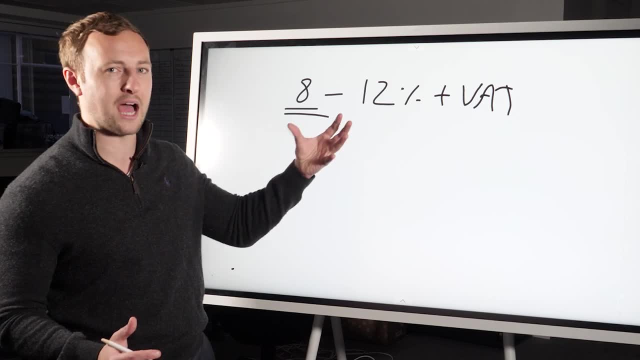 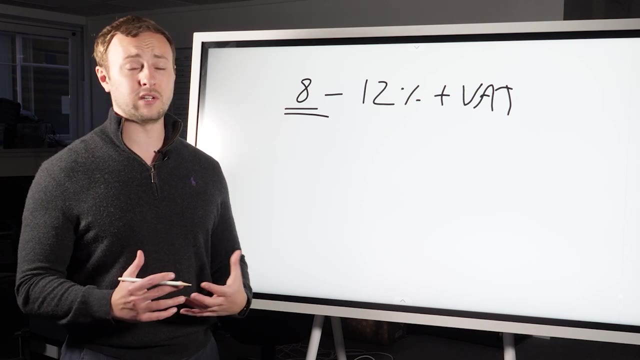 I don't pay 8% for mine at all. I pay more money than that And I'll tell you where I'm paying in a moment actually, because it will help you understand my principles and how it comes around to it. My experience of 8% people is they do the bare minimum. They're not proactively looking. 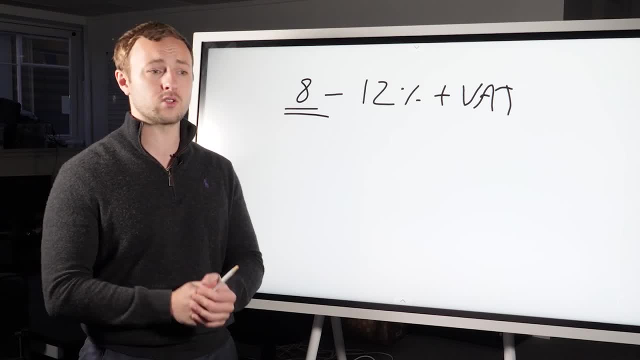 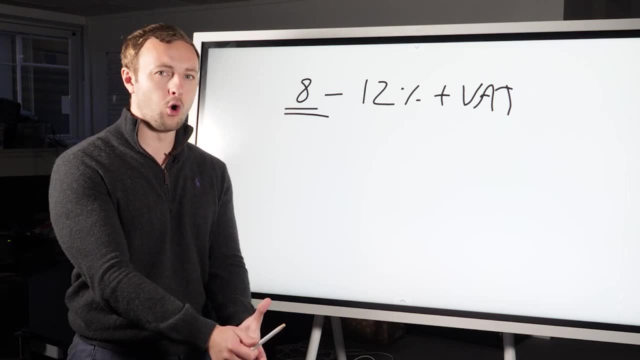 looking to do an amazing job to look after the tenants, to add value to your tenants- which ultimately, by the way, you want, I get that it's an investment, but actually it might be your house, but it's their home And if you can make it an amazing home for them, they're more than likely to treat it that way, spend money on it and stay there for a lot longer And, ultimately, if you've got somebody that's outsourcing everything and it's an online agent, usually doesn't work well for me. Just my personal opinion. 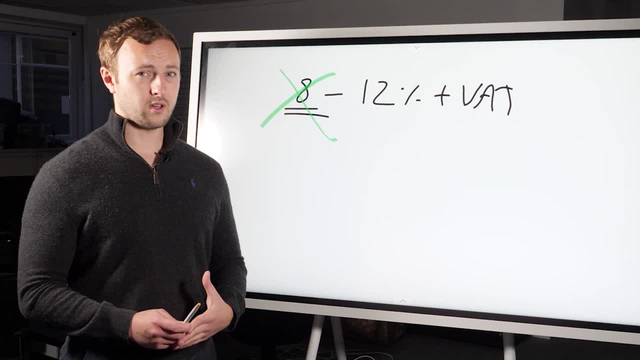 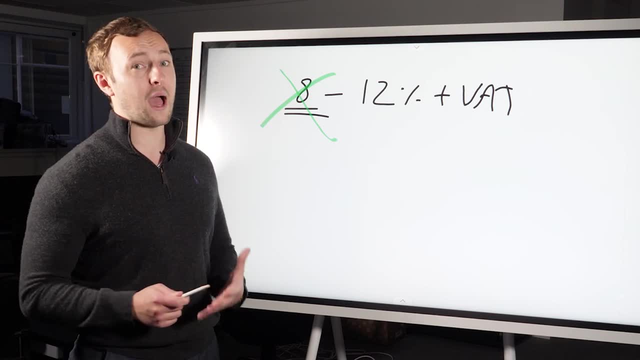 12% for me is a 12% for me is a little bit too much. Okay, I think it's asking for a lot because most buy-to-lets, if you've got a good buy-to-let, doesn't really require that much effort If you've got great tenants in there. 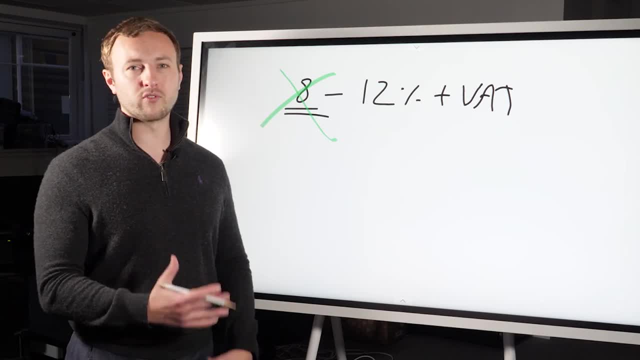 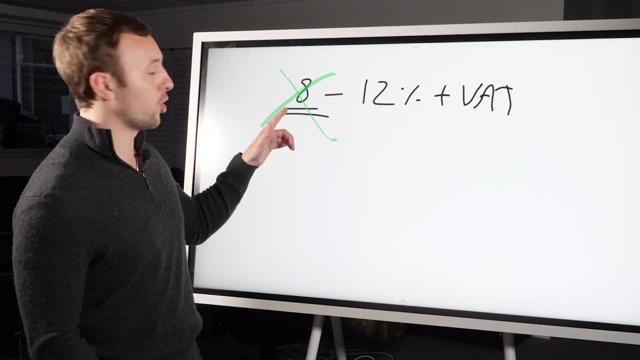 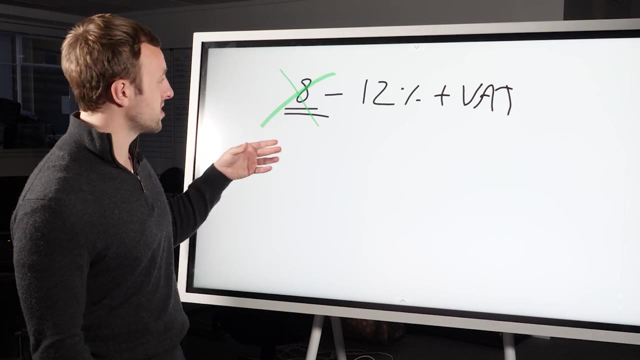 let me tell you what I end up doing. So, because of the portfolio that we've got- and we've got a modest but sizable portfolio enough to negotiate on positions is I know my agents would go to 8% if I put all of my portfolio with them. Okay, Now it's a great negotiation price and it's 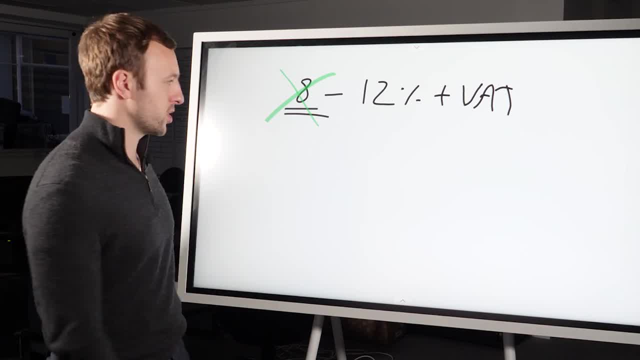 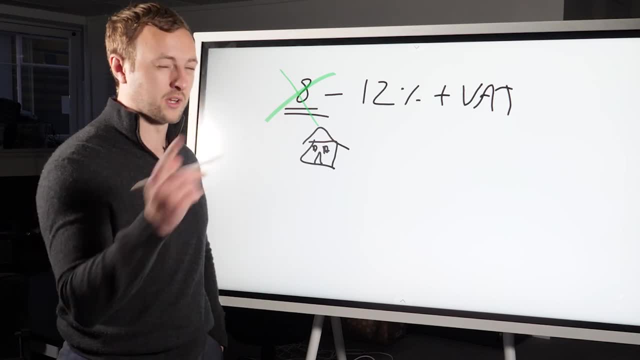 a great deal, a great deal for them as well. But let's just think about this logically: If there's a house what an agent doesn't do- and this is where you might want to consider, and I'll link back to why- 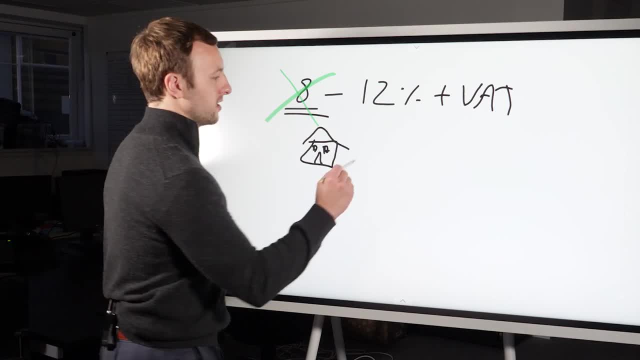 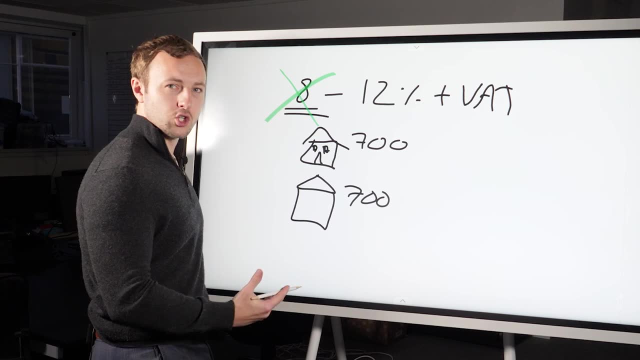 you wouldn't want to use one If there's a house that's there and it's 700 pounds a month, and then there's another house here for 700 pounds a month but the agent is letting it out, And on this one, 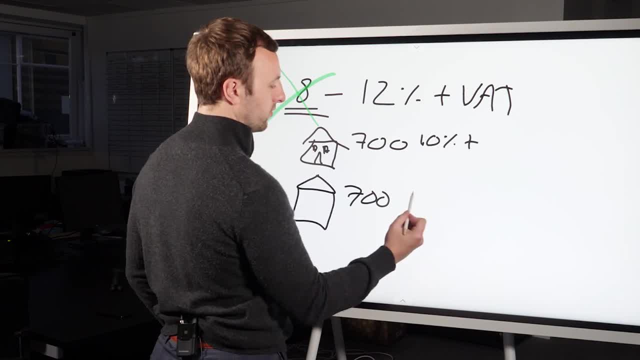 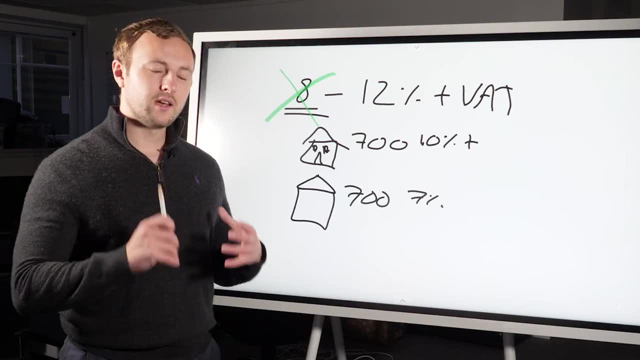 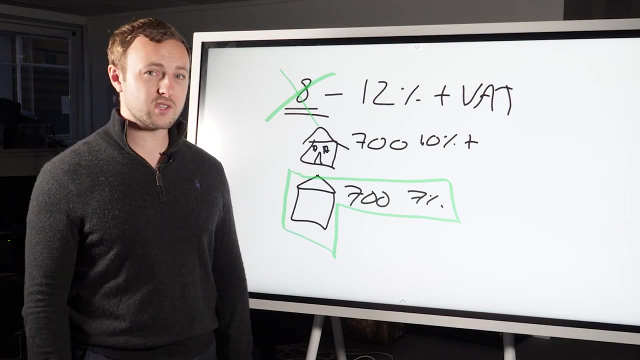 they're getting. you know, let's say, 10% plus, but on this one they're getting 7%. Well, not plus 7%. Logically speaking, even on a subconscious level, what are they going to be doing more of and focused on? Is it going to be the 7% one that they're getting, or is it going? 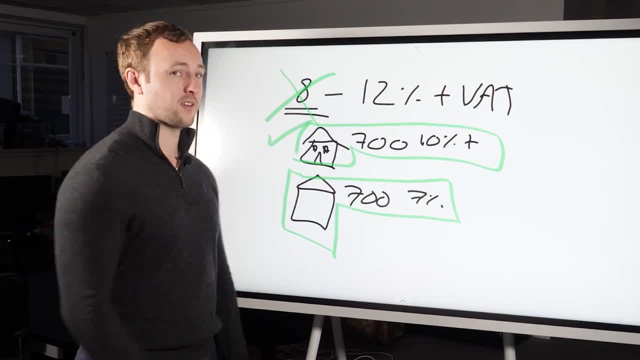 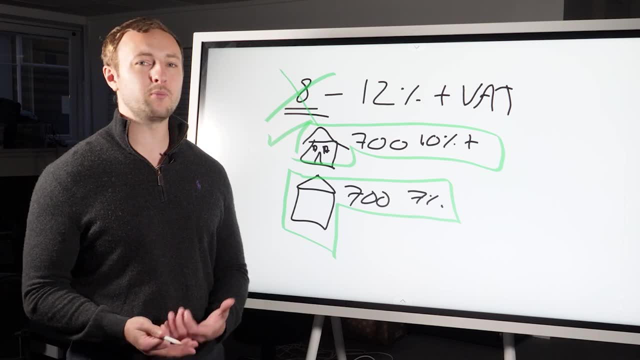 to be the one. they're getting 10%. Hopefully you said: well, logically, it's going to be 10%, And you might be thinking, no, surely not, Cause they're going to show people around. though, Look, people aren't stupid. People are money motivated by money. There's, if there is a loophole. 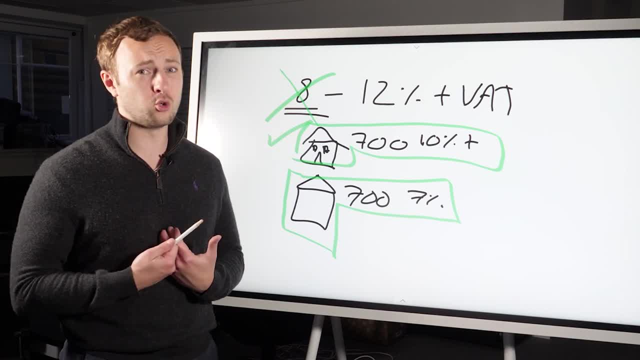 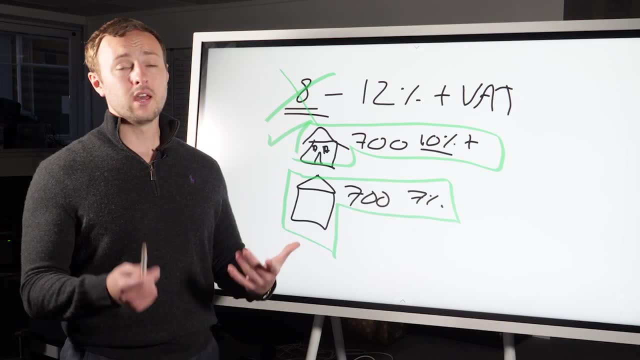 they will take care of it because they're salespeople. I definitely do. Why wouldn't you right? You go for the path of least resistance and the path that's going to make you more money. So if I were a letting agent and I knew I've got five properties on the books, but this one pays, 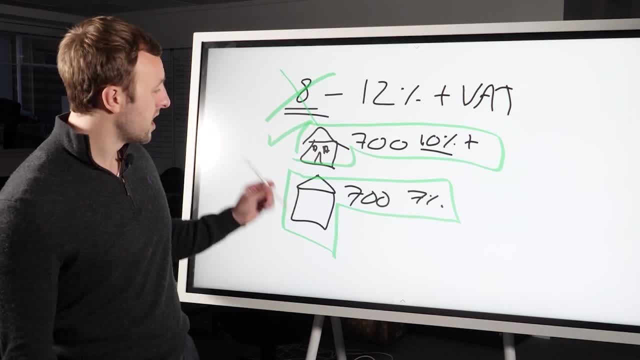 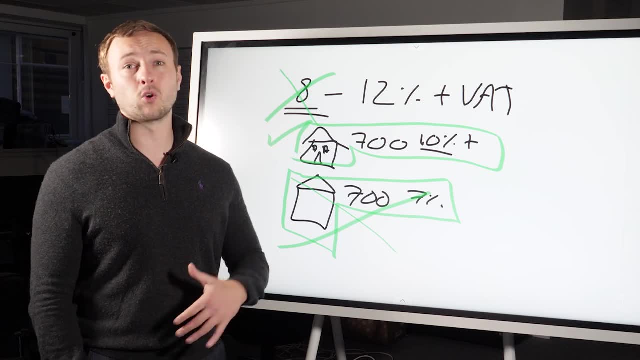 me really well. I love the landlord. They look after me, they give us treats, And then there's all of the other people that all they care about is getting our prices down. I know I'm going to be going to the tenant- Hey look, I've got an amazing property. We've not even put it on yet. 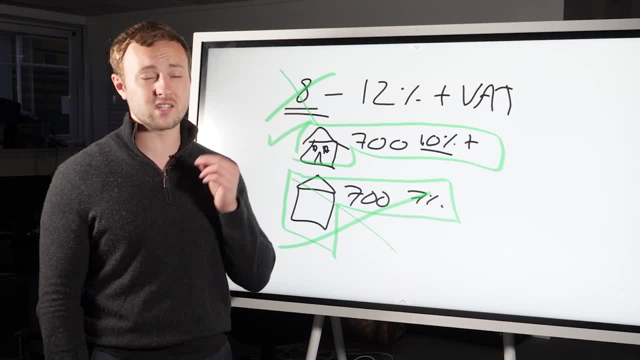 If we haven't put it on, but you're going to want to see this one first. It's in such high demand. That's the one I'm going to take tenants to first. That's the one I'm really going to make. 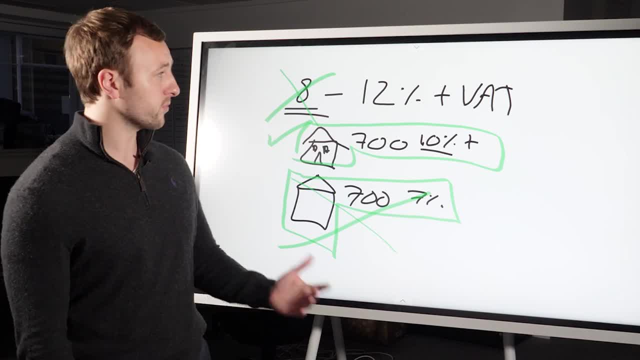 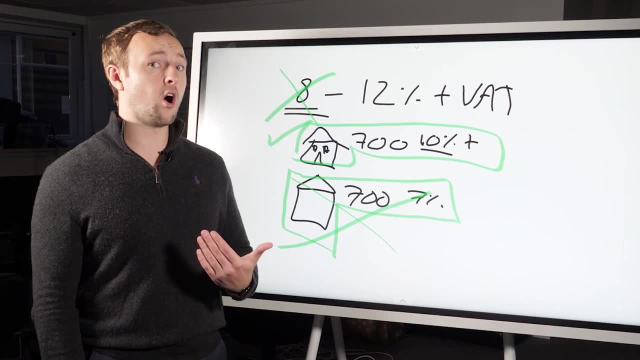 an effort selling and getting them to sign up on the spot, right there. So to give you an idea of what we pay, we typically pay 11% plus VAT for our rentals. That is higher than average for the area, but I don't mind paying it. I think they're exceptional at what they do. They add a 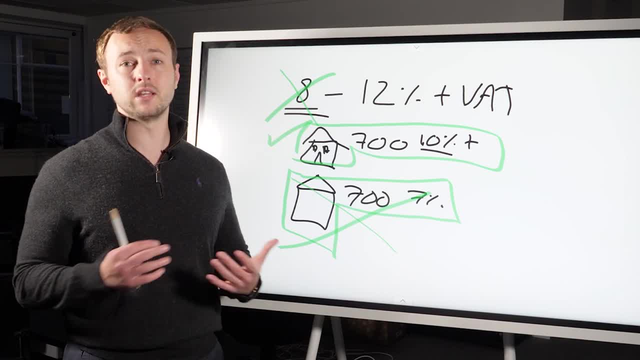 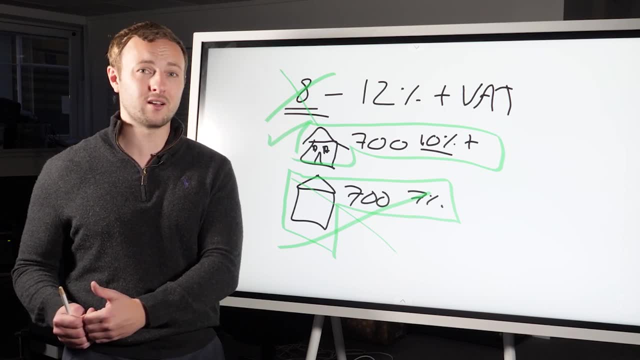 a massive amount of value and service to us And I never need to hear about my properties unless it's absolute necessary And in my experience I've had really bad letting agents in the in the past and man property managers And it just goes tits up and the properties just aren't well. 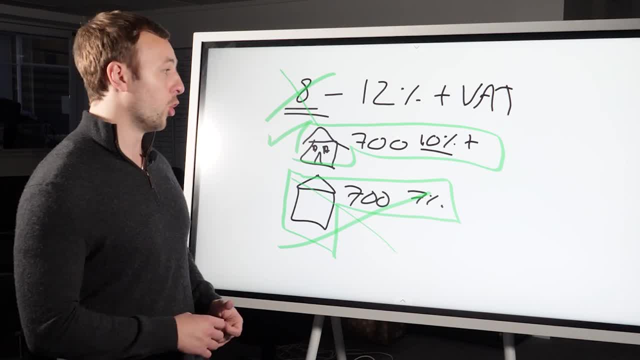 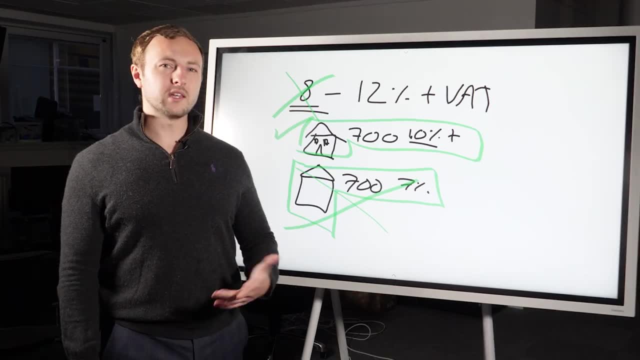 maintained, They don't have the inspections and things start to go wrong And ultimately, the value from your property is over the long term, not just the next five to 12 months. Okay. So with that in mind, it is important to understand. let's say, let's go with 10%, because 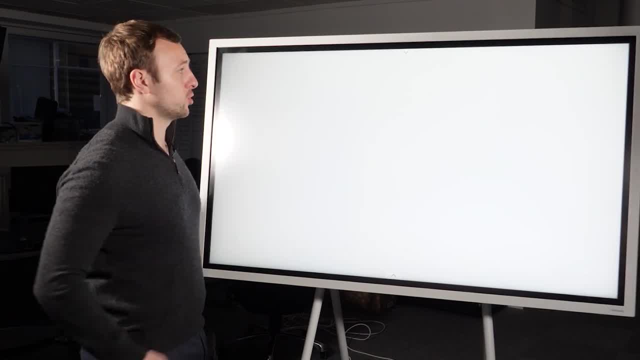 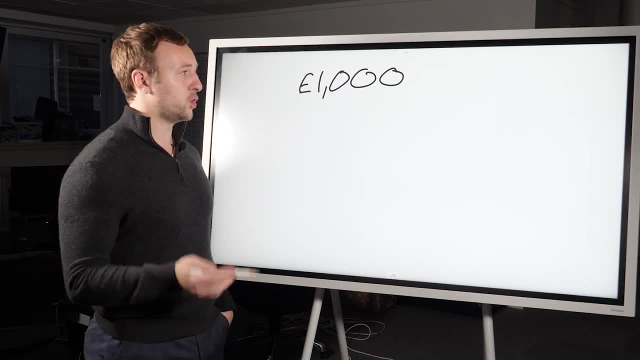 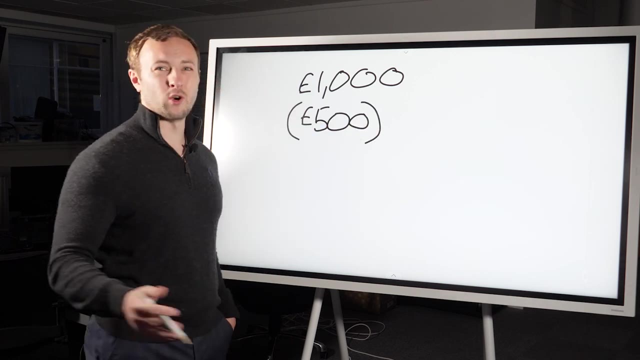 this is where a lot of your profit is going to go. Okay, And I'll do, For example with a thousand pounds. I know it might not be representative of a rental in your area, but if you factor in, let's say, you've got 500 pounds worth of costs on this, which is pretty. 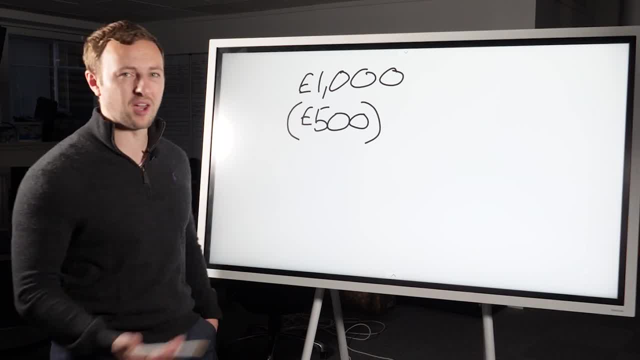 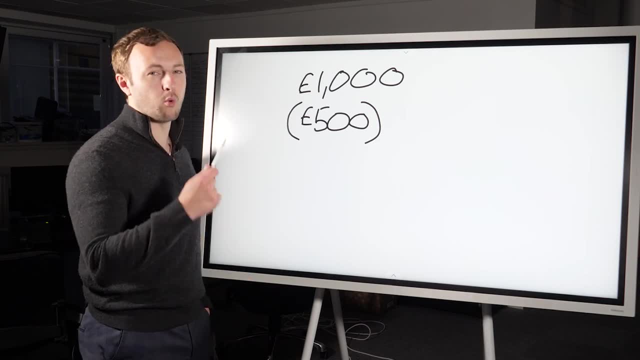 typical. it's going to be your mortgage, your voyage, your maintenance, whatever. it might even be a bit higher, but just bear with me here. If you've got 10% plus VAT on there- and most people aren't VAT registered if they're portfolio builders, some of you will be, which is great. 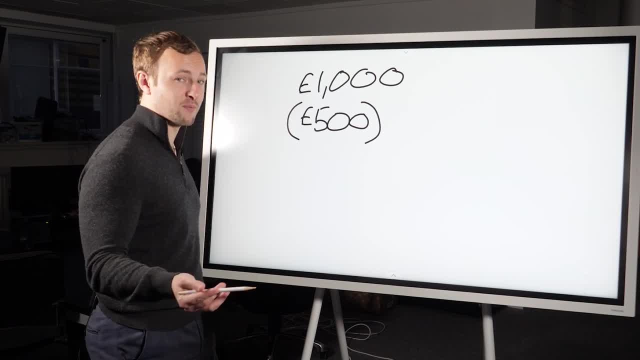 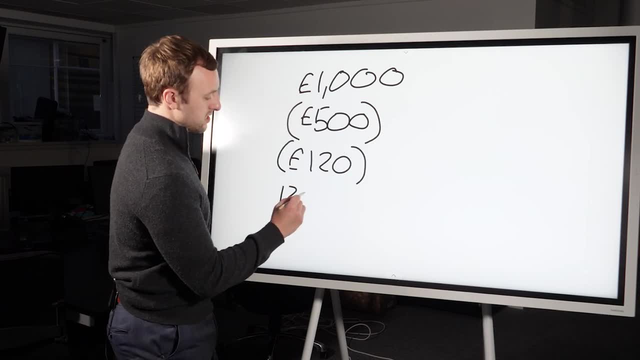 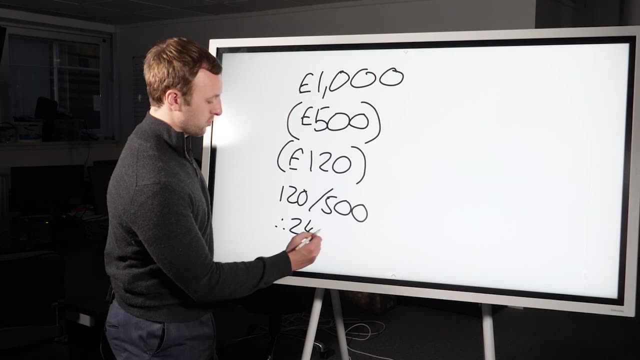 That's going to be 10% plus VAT, which is the equivalent of 12%. That's going to be 120 pounds. Okay Now, 120 out of your 500 pounds. profit is almost 25%. It's around 24% of it. Okay, That for. 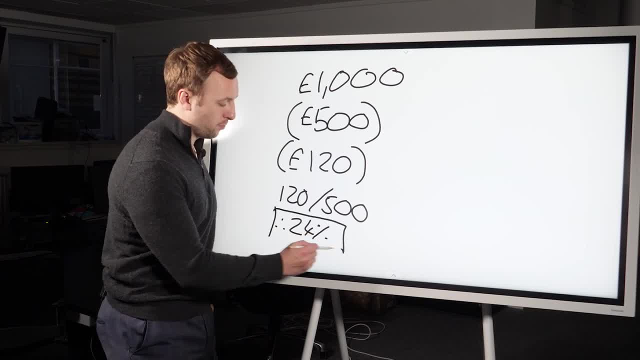 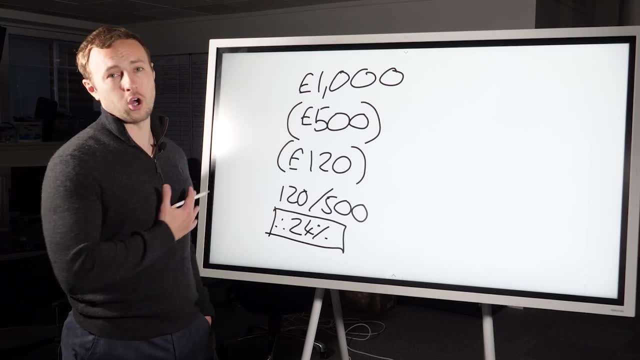 me is absolutely staggering. So 24% of your profit has just gone paying somebody else to do that For me. it's worthwhile. 20% of the profit is just going to be me, which at the moment it's not that it's really worthwhile. 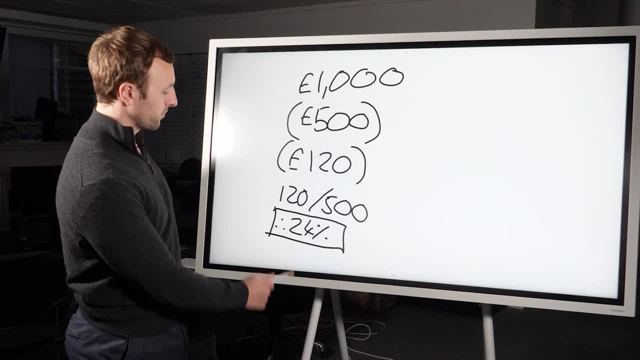 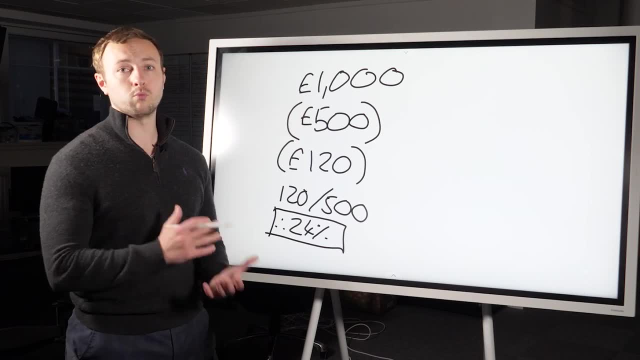 It's not that it's not going to be that. that's the problem, because you know it's a short term gig which I'll get to in the down the line, but it's really worth thinking about with that cost going out. So are there alternatives? Would I just not use them? Well, yes And no, if I were local to. 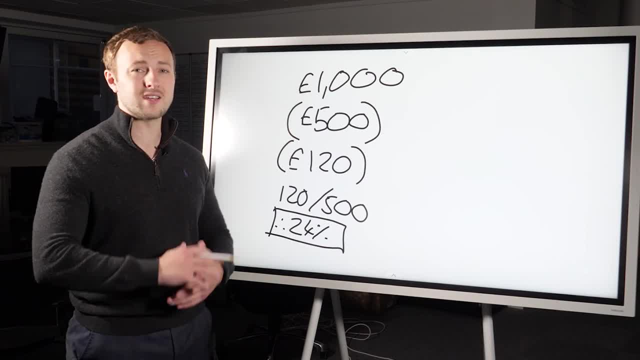 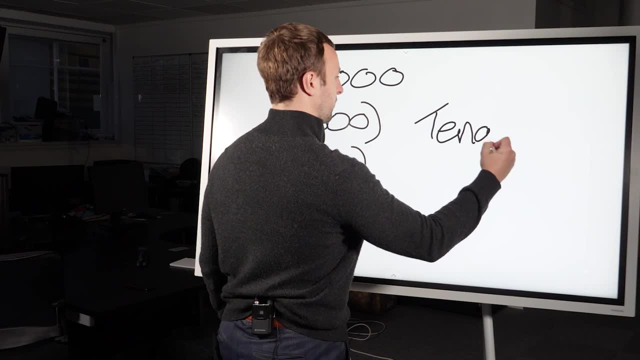 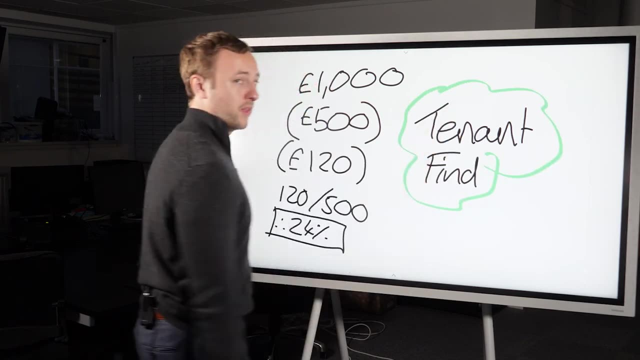 my property and it's a well refurbished property and I know it's going to attract great tenants into this property. what I would personally be more drawn to is a tenant find. a tenant find is when an agent will go out there and do all of the necessary checks at the beginning. okay. 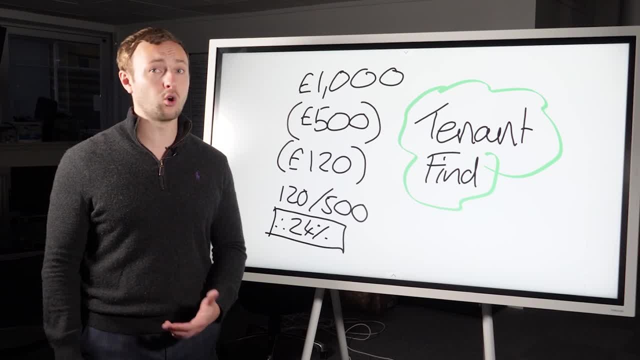 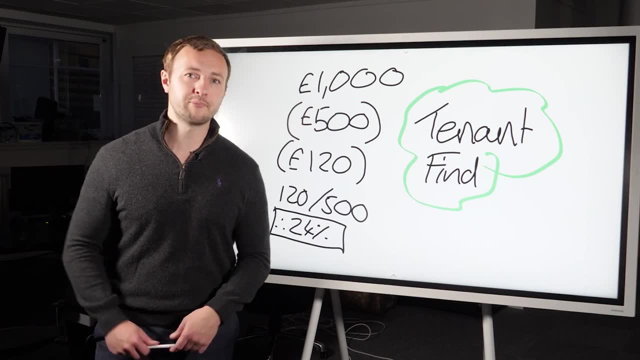 now they are going to charge you for this and it will be a decent chunk of the month's money and usually it's three to four weeks, but you can negotiate that, dependent on your area, probably about 500 pounds. okay now, the reason i really like tenant fines is there's a lot of 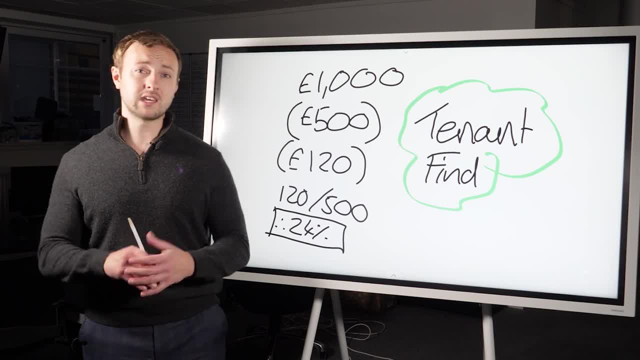 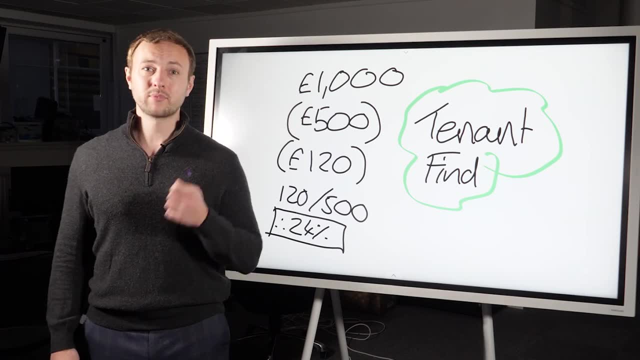 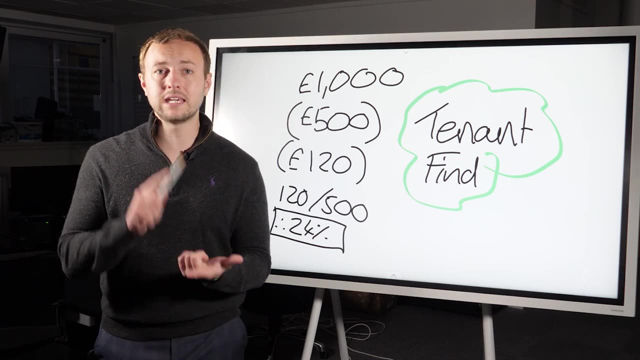 regulation you might not be aware of when taking in a property and you usually don't care about it until you're getting a tenant out of your property, and i'm going to explain. if a tenant moves in and they haven't been given the correct ast um an e a copy of the 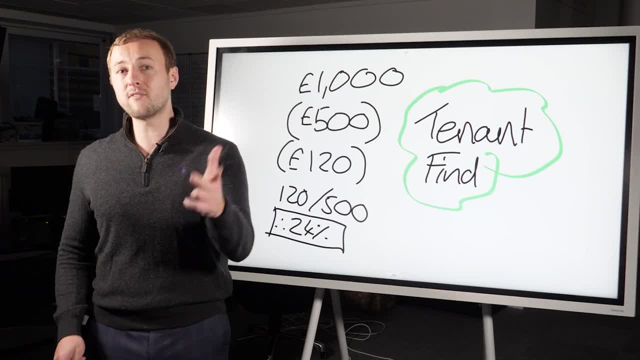 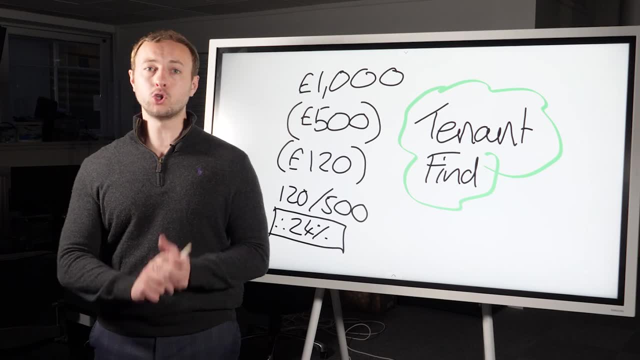 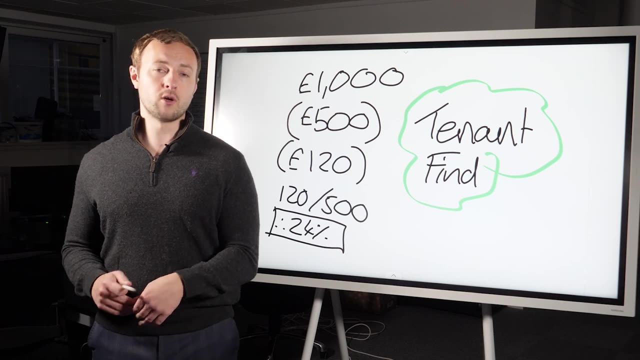 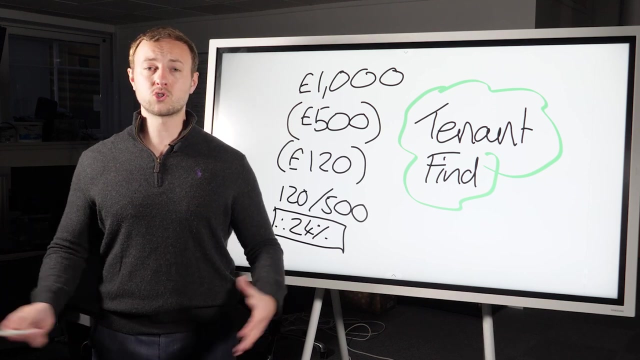 epc- the energy performance certificate- if they haven't signed a document and read over the terms of the letter agreement and the right to rent guide for the uk. right now it is not always, but almost always, illegal to serve them with a section 21 notice or a form of notice to kick them out of your property. so, for example- not that you'd want- 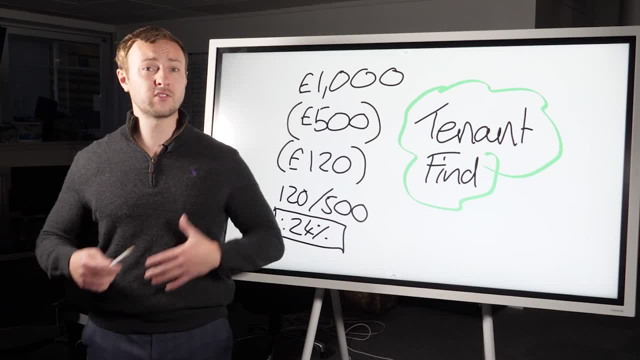 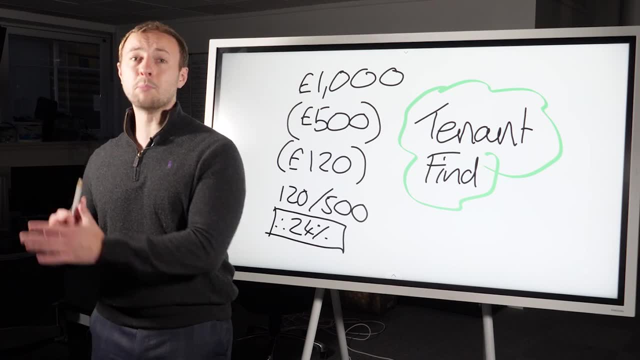 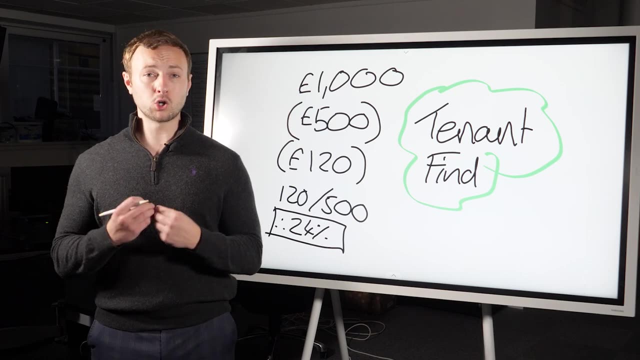 to, but if a tenant was causing a load of issues down the line, if they weren't paying you and you wanted to evict the tenant, it is so much harder to near impossible to do if you didn't get that documentation right in the first place, and for me, i'd much rather not take that liability on. 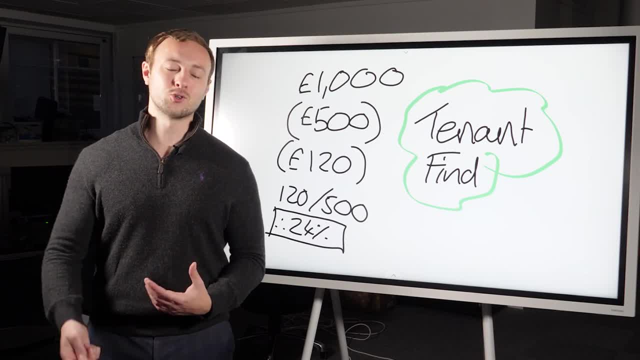 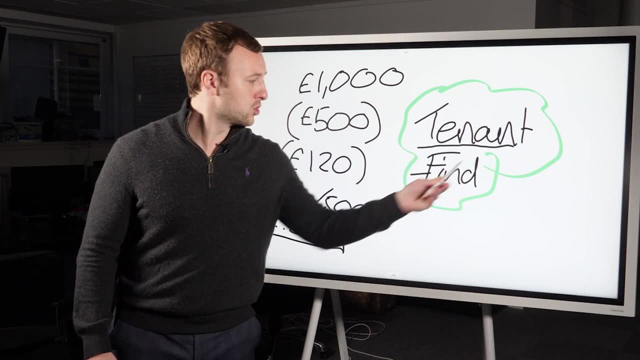 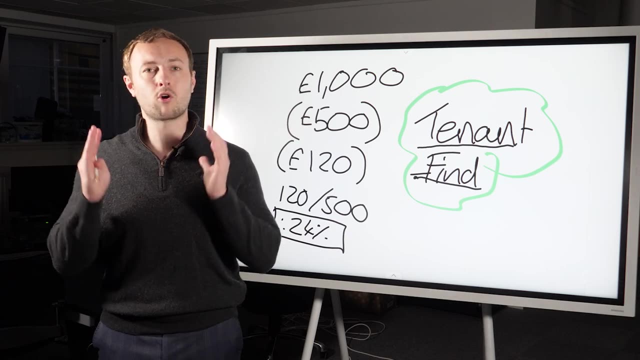 and of course i'm the owner of the property, i am the landlord, so it always falls down to me with that liability. but ultimately i would prefer to pay somebody separate to go out there and do that tenant find and take that liability and obligation to themselves and give them a strict criteria. 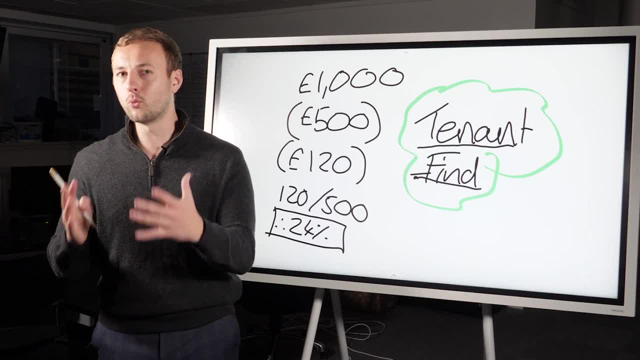 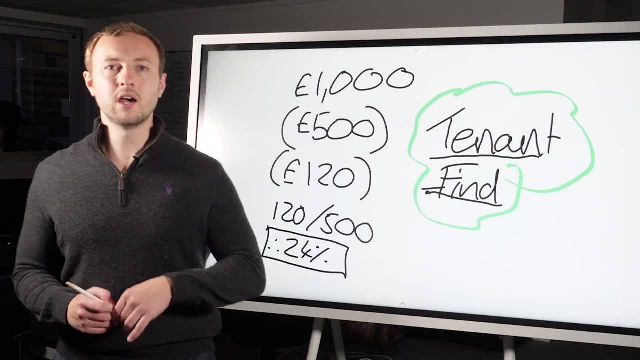 of exactly the type of tenant, within the boundaries of the law, that we can say that we want in our properties. so, again, i'd only do this if the property were local to me and i'd want to build a relationship with that person, and if you've got a great relationship with two or three. 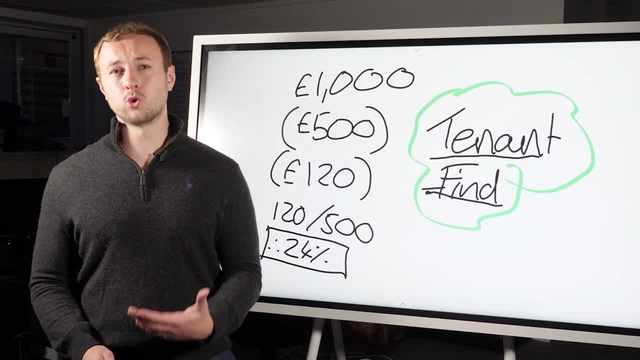 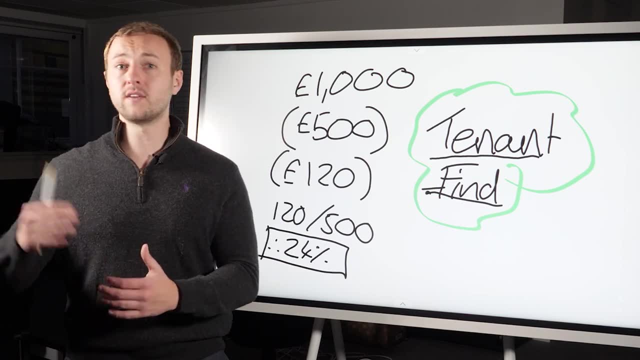 tenants. as long as they don't have a property, they're not going to be able to take that liability and if they don't take the mick normally, it's absolutely fine to self-manage. however, if you're looking to do this, to scout a big portfolio, and you want 10, 20, 30, 50, 100, 200 properties which by 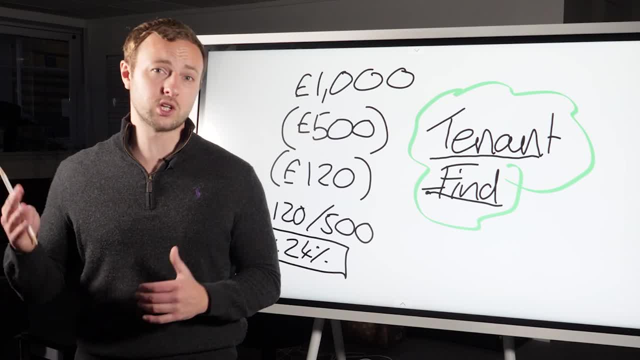 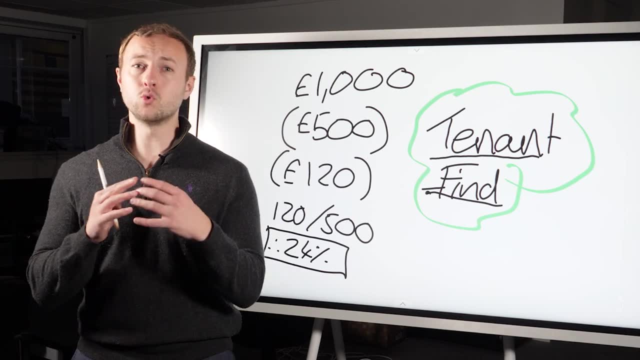 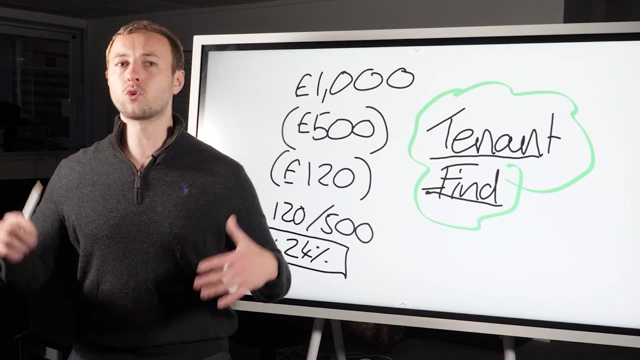 the way might sound crazy for some of you, but it's definitely potentially possible over your lifetime to get over 100 properties outsource. in the meantime, okay, just utilize other people's time, take the headache away from yourself and focus on your growth. i prefer to spend my time. 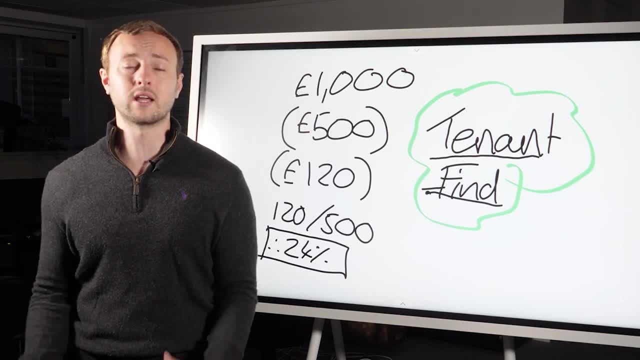 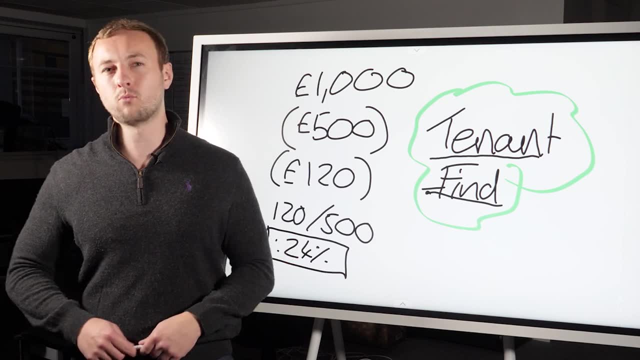 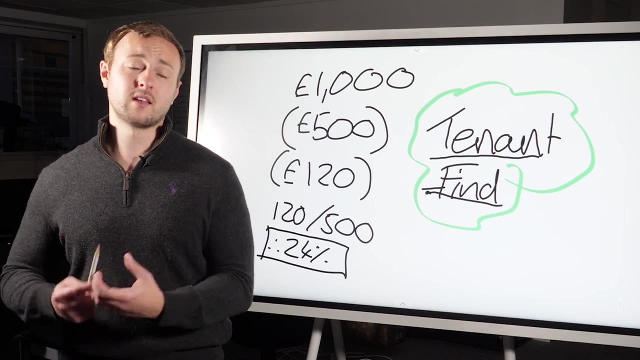 focusing on marketing, focusing on putting myself out there, focusing on increasing my active income and utilizing that active income to purchase more property rather than worry- worried about 30, 40, 50 quid in the background, which is more typical of our management fees, um and and focus on growing. 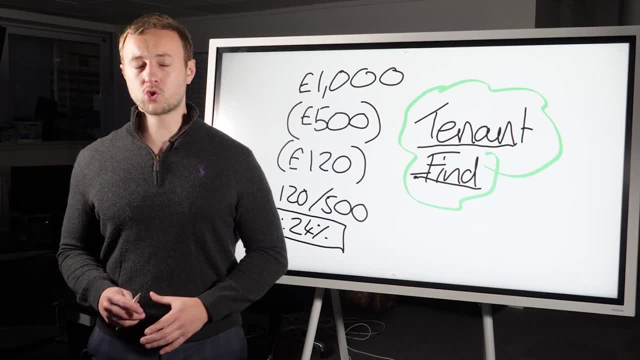 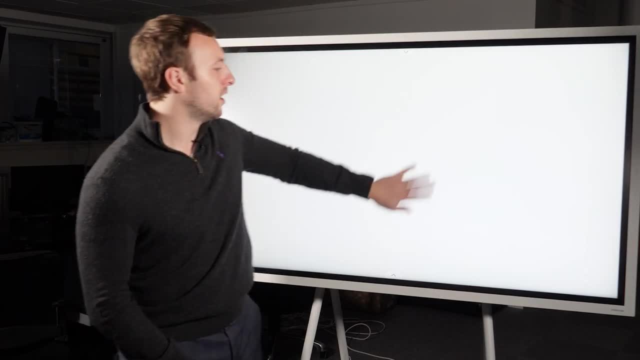 that portfolio. so i just want to give my final thoughts on this, on how you take it a step further, because stage one might be the situation where you know what i'm going to use a tenant, find we're going to put tf on there because i want to outsource all of 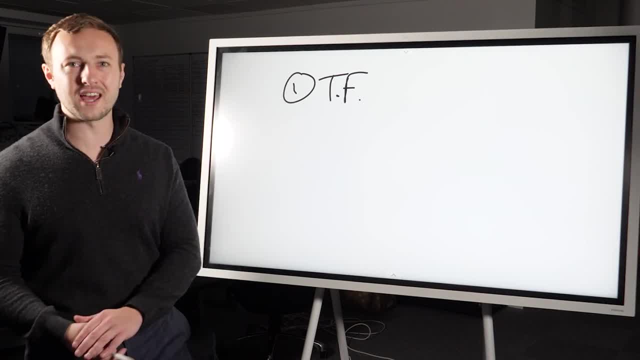 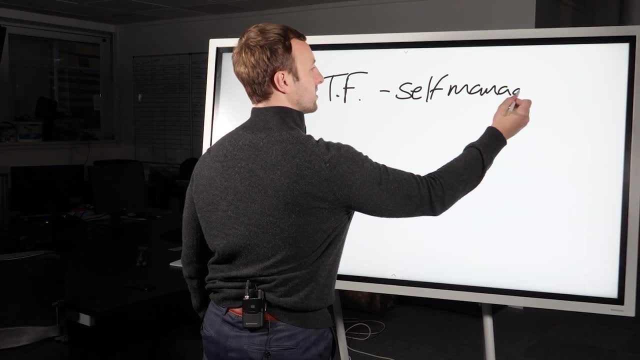 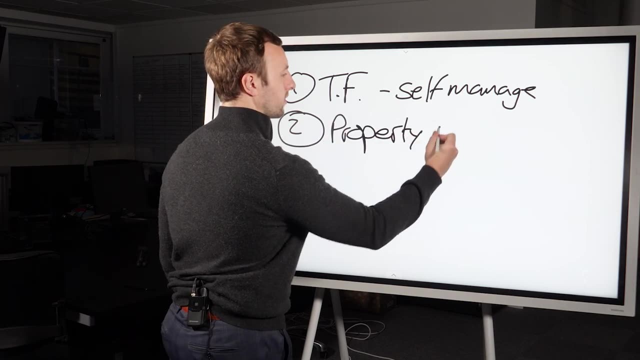 the responsibility and effort of, you know, driving around, showing tenants, around all of that, and then i will self-manage and then what typically happens is it does this sort of full circle, because what we're going to get in place is a property manager and then once we've got that property manager and they're 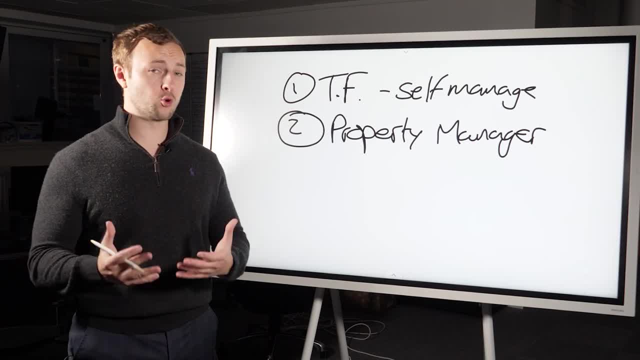 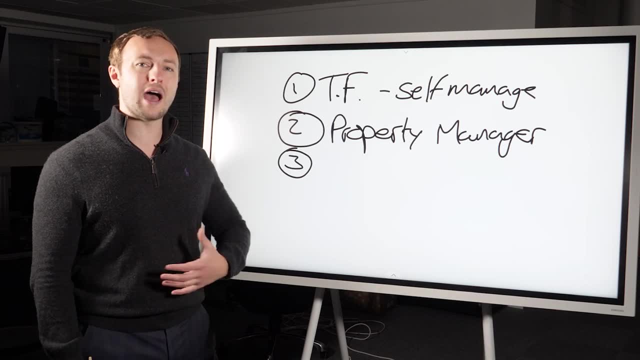 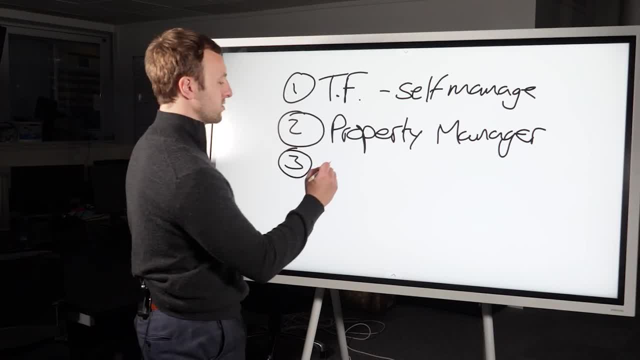 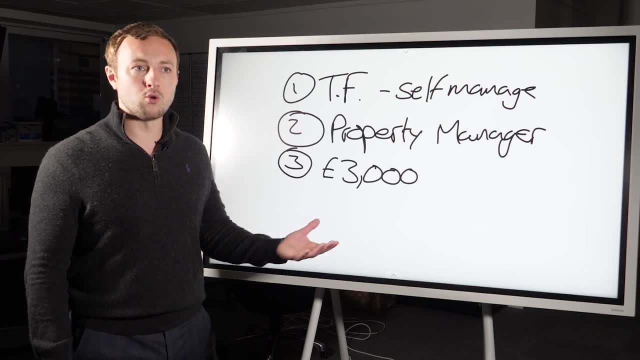 you know, i wouldn't do this at a break-even point, but maybe at 3 000 pounds, something like that, of a very rough estimate, which might not well, it is a lot of money, right? so let's say you've got um properties where the rent is. 750 pounds. that means let's scrap the v80. just to make this simple, you're getting charged 10 of 750 pounds, so 75 pounds per property. that's coming into this, that's going to be 40 properties. 40 times 75 is 3 000 pounds.